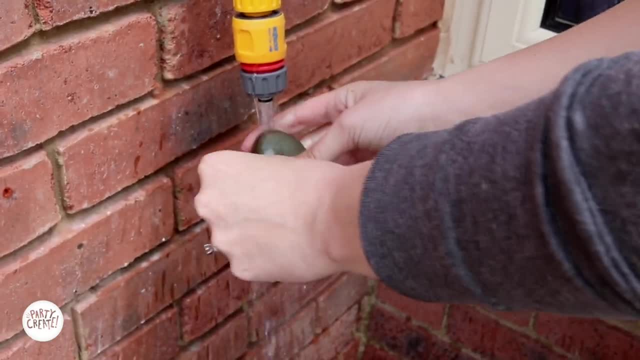 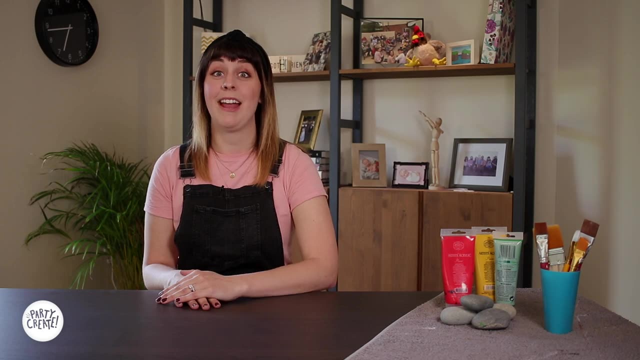 So it's really important that you make sure your rock is nice and clean before you start to paint. We also put our rocks outside in the sun after we washed them. That way, they got nice and dry before we started. Now this part is really really fun. This is the. 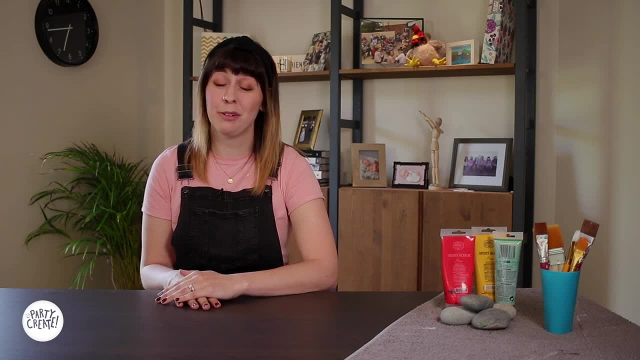 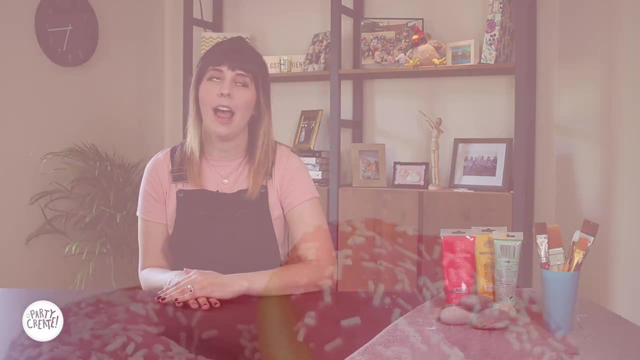 part where we get to decide what we're going to create. Now, since we've been on lockdown, I've been missing out on a lot of my favorite things, And one of those favorite things are donuts. I love donuts, So what I'm going to paint is a strawberry donut. Now you can paint whatever. 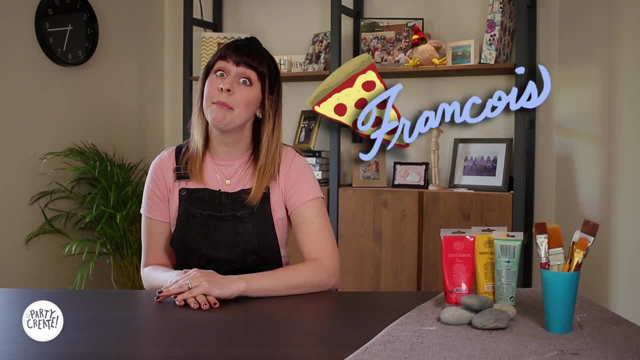 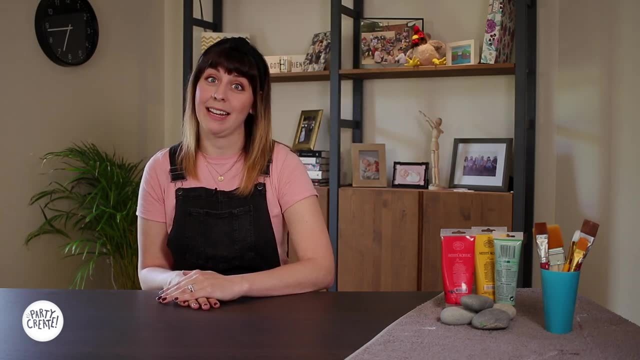 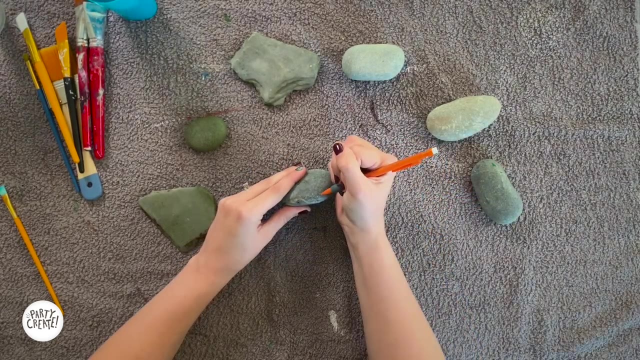 you like. You could also paint your favorite food. You could paint your name, You could paint your person on TV, Pretty much anything you want. Now let's start creating. Now that we've decided what we want to create, we're going to draw it on our rock. So, because I'm making a donut, I need to take 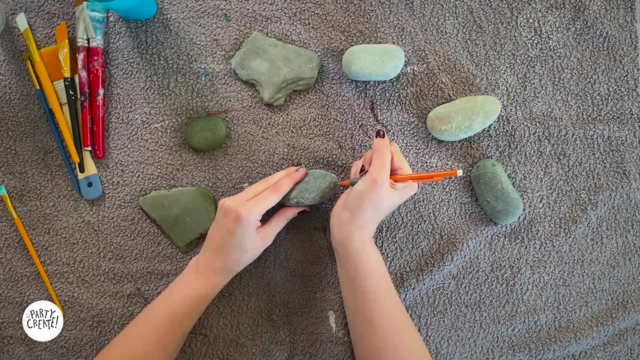 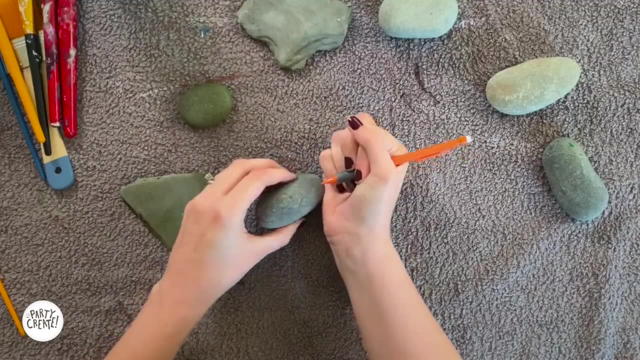 some time drawing some really nice lines for the icing. So I'm going to draw the icing all around my rock like this, just like so. So that way, when I get my paint out, I know exactly where to make all my lines stop. 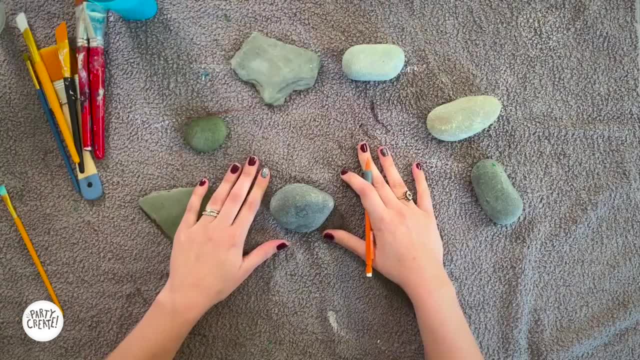 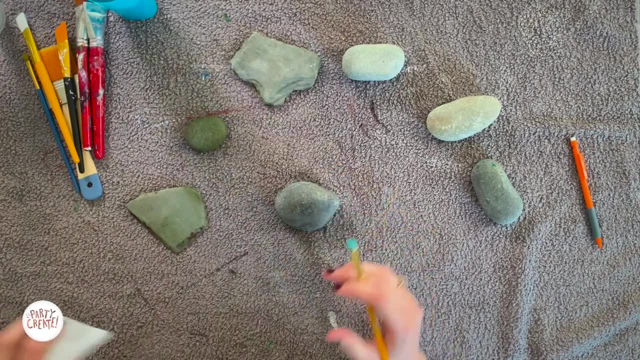 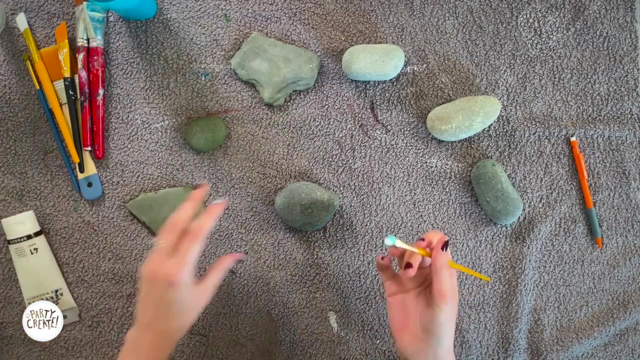 So there's my icing line. So now we've drawn on where our icing's going to go and we know where to put our base coat. So for mine I did about three different base coats, So I'm going to take my white paint before I put on my pink paint. That way the pink will really pop, If you're. 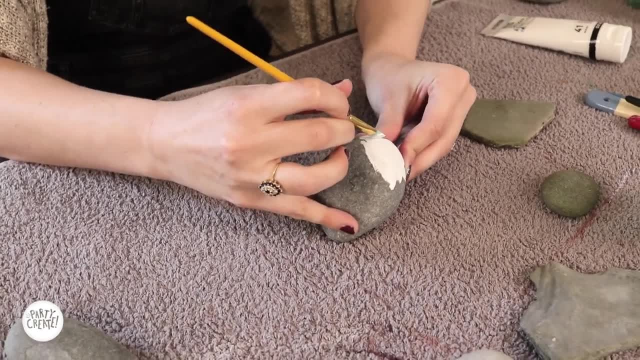 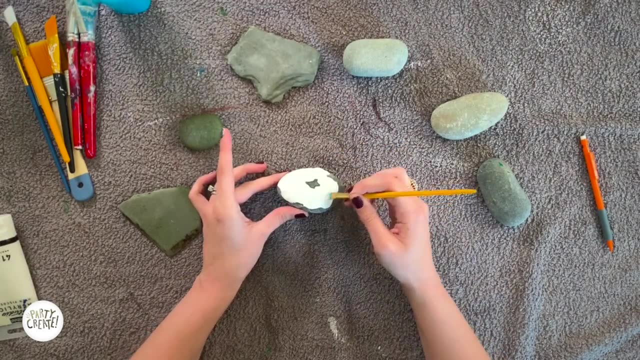 doing something different. you might want to do a black base coat or a different color base coat, but I chose white because I think when I put the pink on top, the white is really going to make that pink strawberry. So I'm going to take my pink paint and put it on top of my pink base coat. So that way, my pink 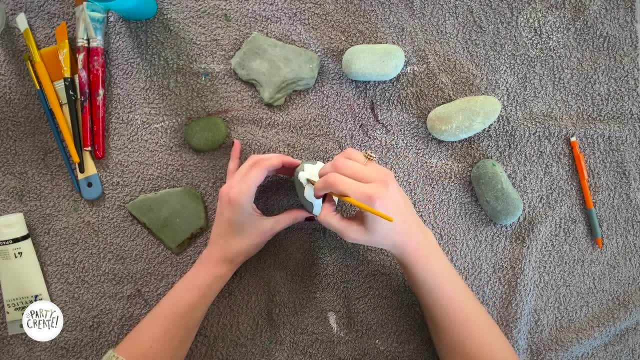 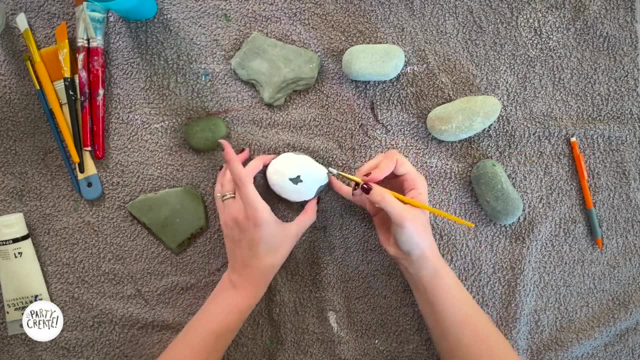 color and the icing look really, really bright. So now that I'm almost done with my first base coat, when I'm done, I'm going to let it dry for just a few minutes out in the sun And then I'm going to 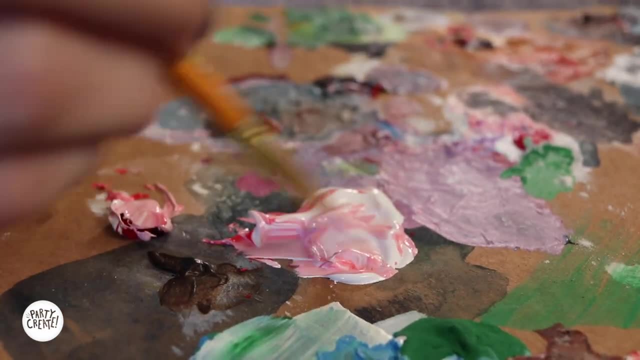 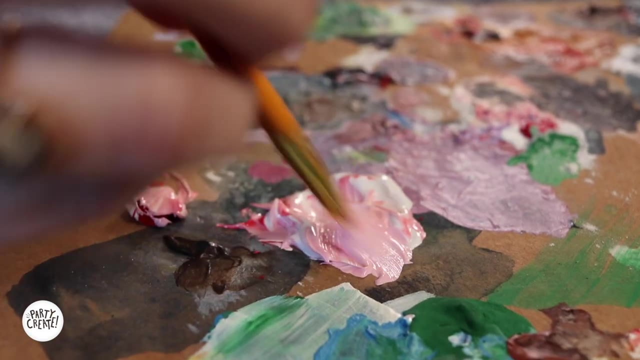 put on another layer of paint. I'm going to repeat this base coat process three times In order for me to make my strawberry color. I took two parts white paint and one part red paint, And let's see how this pink comes out. 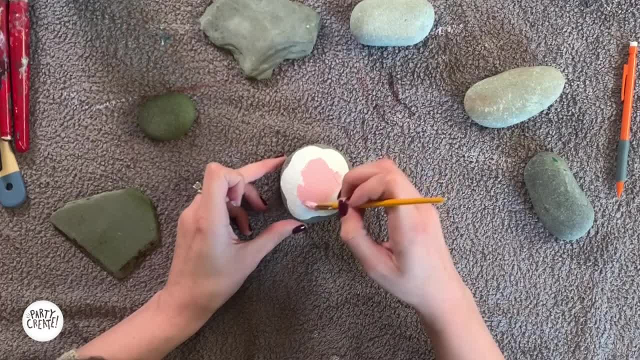 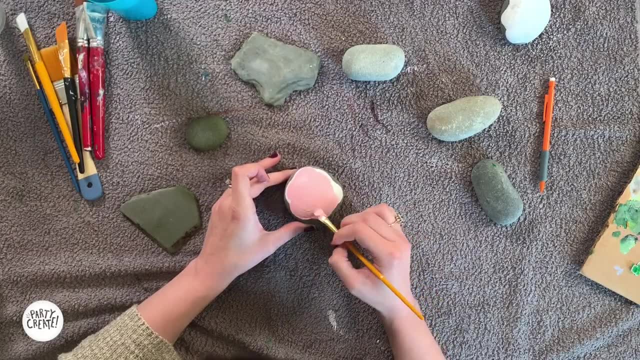 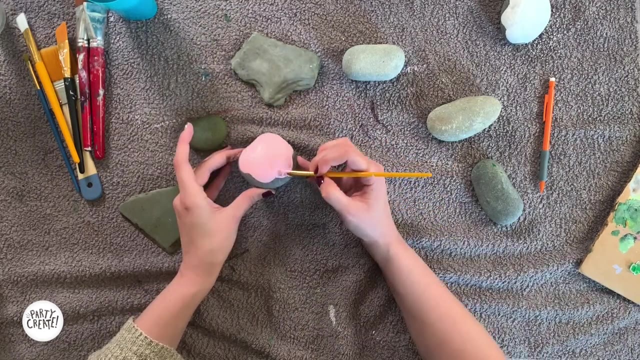 Oh, look at that, Yum. So I'm just putting right, putting it right over my white base coat that I did just like that. So it looks like some really good strawberry icing. Now that we have our icing done, we're going to let this one dry for just a few minutes before. 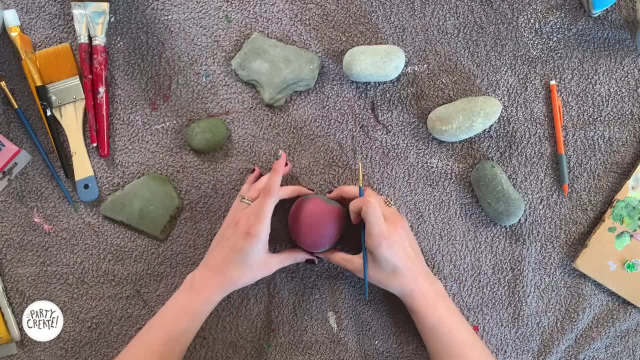 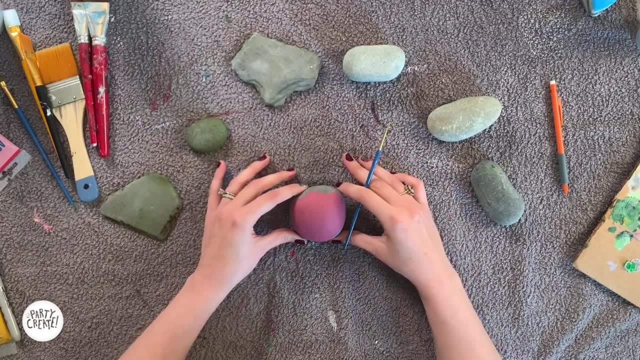 we put on our sprinkles, So I made my icing just a little bit darker. And now that that is all done, it's time to do some sprinkles. This is super easy. All you need is a really thin brush and two colors. 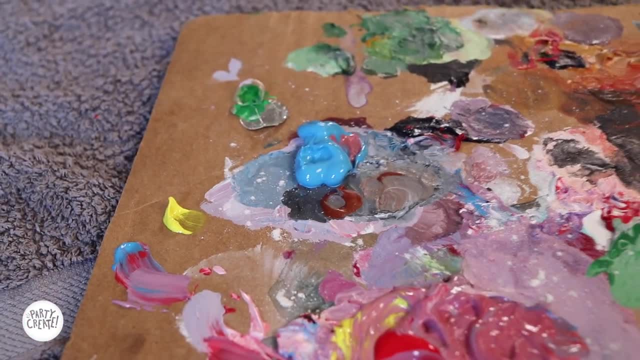 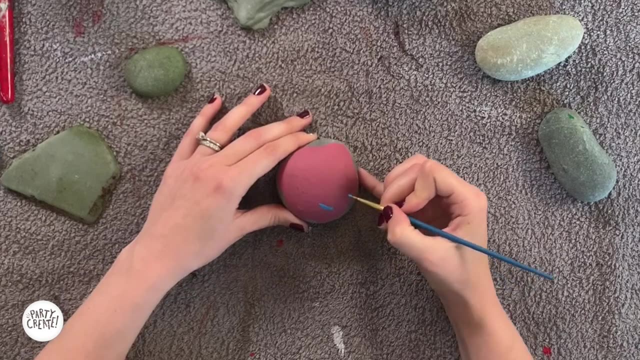 I chose blue and white for my sprinkles, So let's get started. I'm going to take my blue first, And you're just going to want to make really long lines for your sprinkles like this. I really like the blue because it just really pops against the pink. 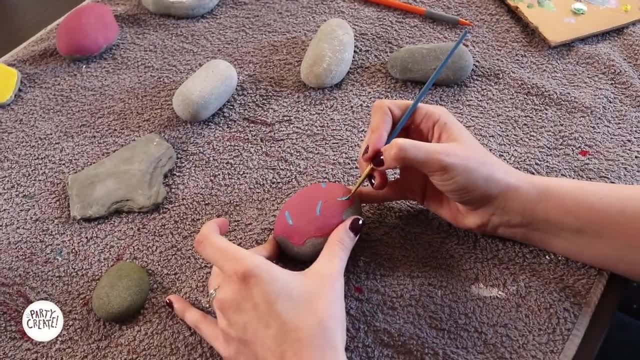 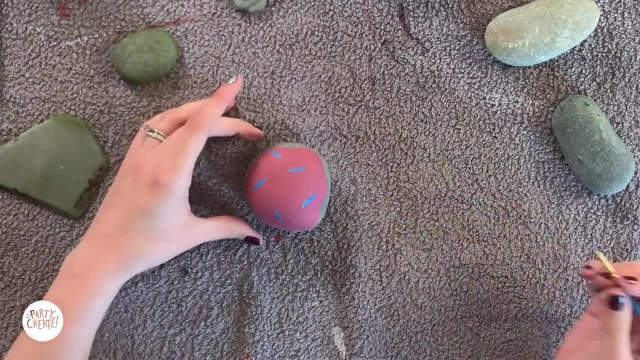 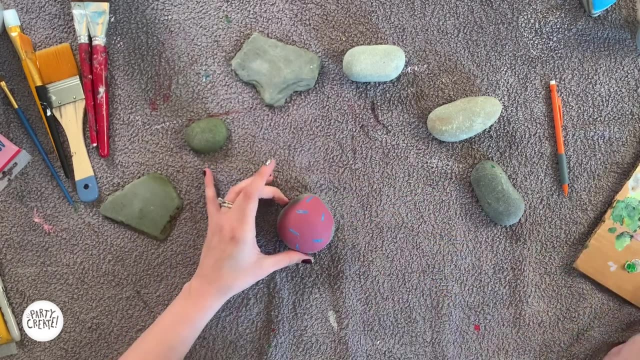 You can just scatter them all over your donut. It doesn't need to be in any specific place. You might want to do two layers, just so your sprinkles show up a little bit better. So now that my blue is all done, I'm going to clean off my brush and my water. 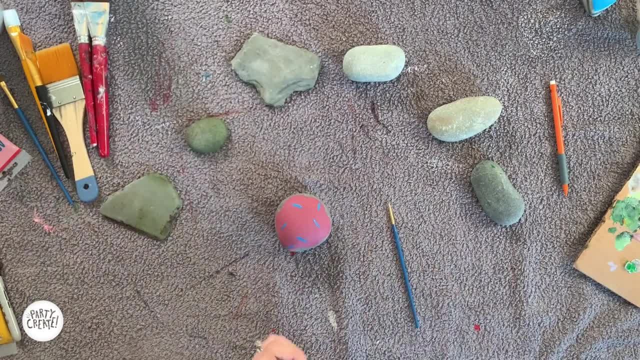 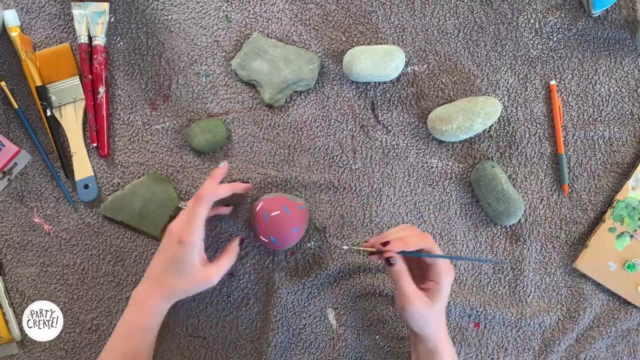 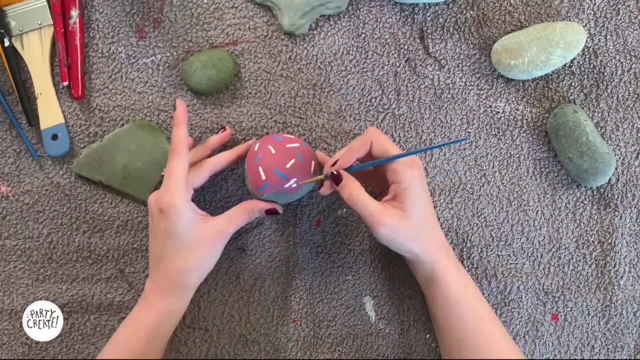 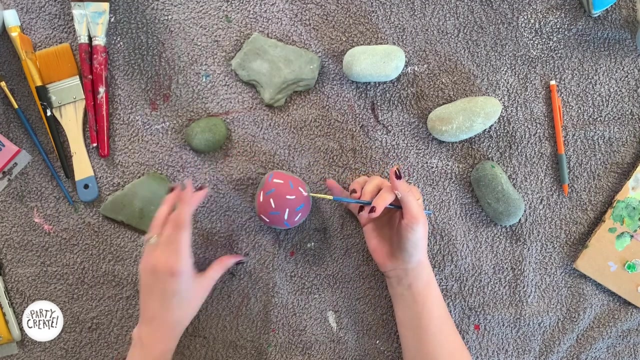 wipe it off on my towel and get ready for some white sprinkles. Yum, Look at that. Now just for our next part. so it pops a little bit more. you can take your small, small paintbrush that you have white paint on, or you can take a. 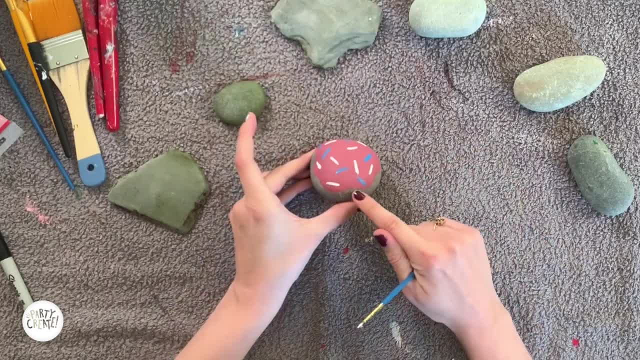 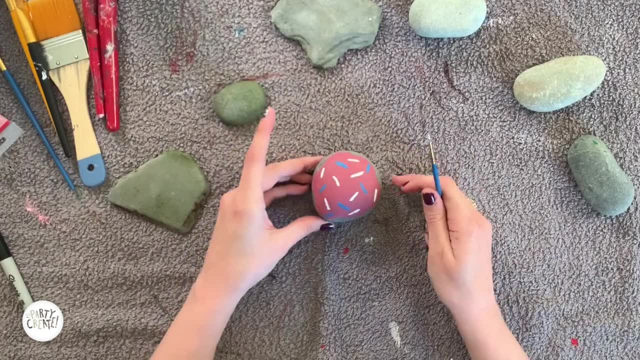 permanent marker, And what I'm going to do is I'm going to take one of these and I'm just going to go around the icing on the outside, against the rock where the icing ends, and just do a really small line, just so the icing really pops. All right, here we go.